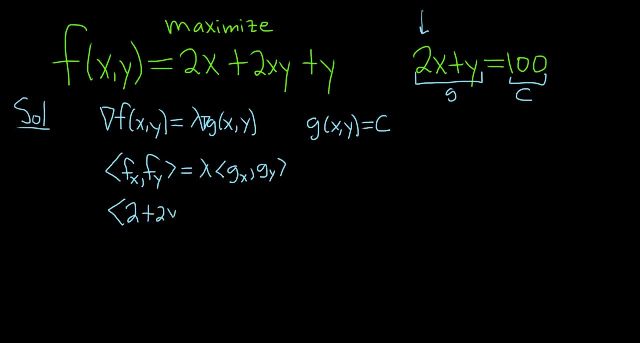 So we're just left with 2y, And the derivative of y is 0, so I won't bother to write it. So comma. Now we have to compute the partial derivative of f with respect to y. Well, the derivative of 2x is 0.. 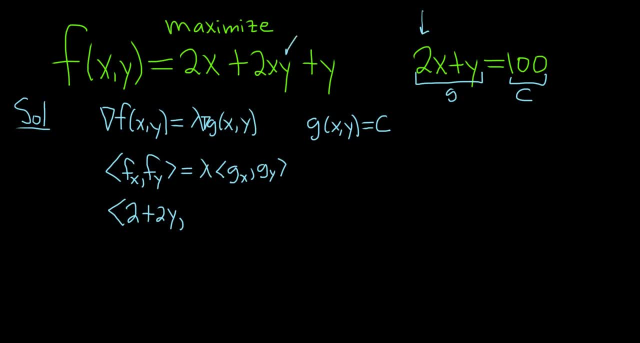 The derivative of 2xy. well, let's think about this: The derivative of y is 1, so we're just left with 2x, And the derivative of y is 1, so plus 1.. That's equal to lambda. 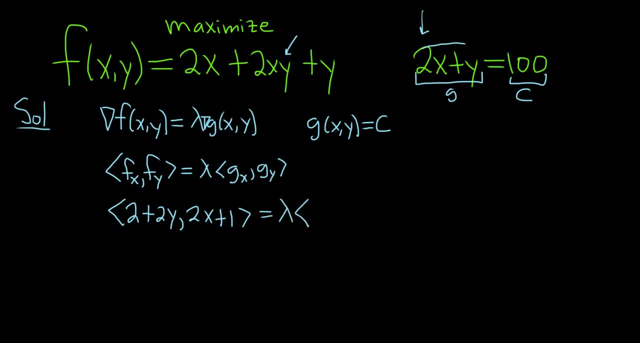 And then we have the partial derivative of g. This is always our g over here, so it's just going to be 2, right, because the derivative of y is 0, and the derivative of 2x is 2.. And the partial derivative of g with respect to y is 1, right. 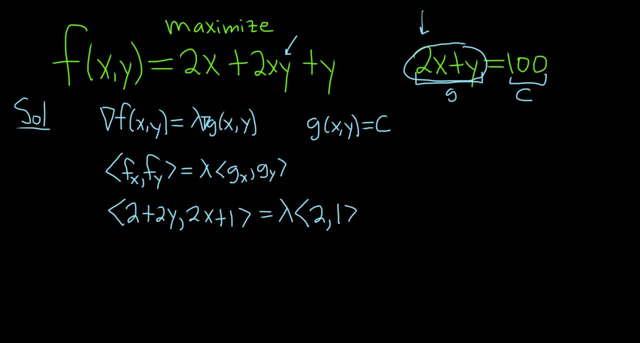 because 2x that goes to 0.. Okay, so we did some math here. So we have 2 plus 2y comma, 2x plus 1. And then we have our angle bracket And that's equal to. 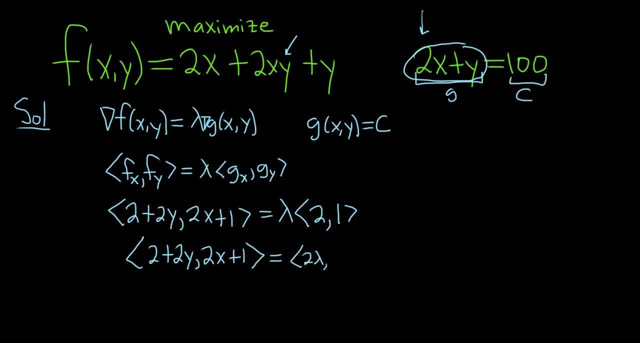 You can distribute, You can distribute the lambda. So this is 2 lambda lambda. All right, good stuff. So these vectors are equal when their components are equal. So we'll take 2 plus 2y and set that equal to 2 lambda. 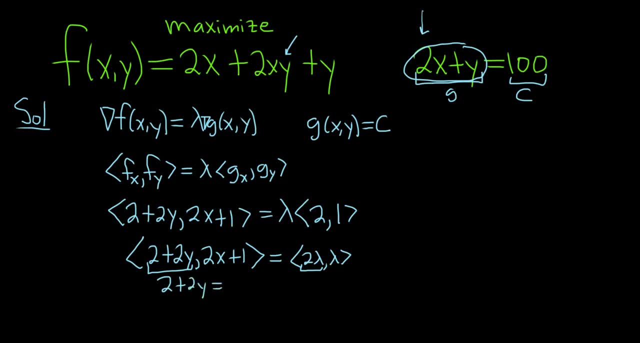 So 2 plus 2y is equal to 2 lambda. Okay, And then we'll take 2x plus 1 and set that equal to lambda. So 2x plus 1, and that's equal to 2 lambda. 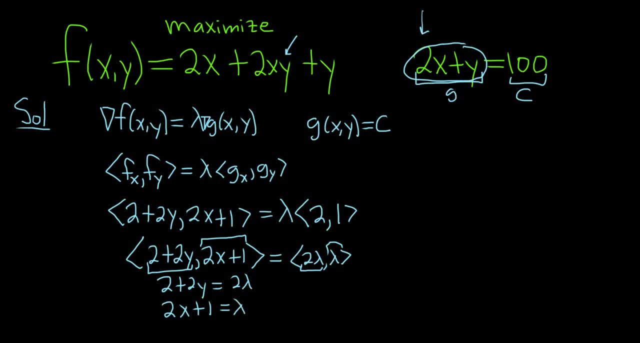 So how do you solve this? Well, it's up to you, but I'm a really big fan of matching. So we have we have like a 2 lambda here. It'd be really nice if this was also a 2 lambda. 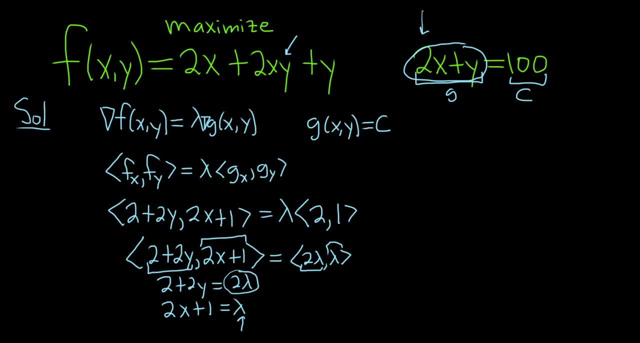 That way we can set these equations equal. So what we can do is we can multiply the bottom equation by 2.. When we do that, we get 2 times 2x, so that's 4x and then 2 times 1,. 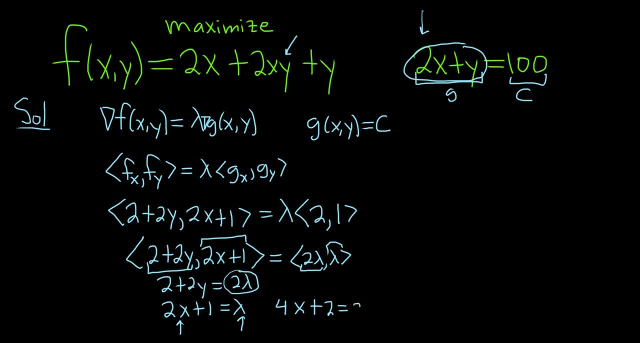 which is 2, and then we get it looks like 2 lambda. right, 2 times lambda is 2 lambda, So this is also 2 lambda. So these are both 2 lambda. That's 2 lambda. Therefore, 2 plus 2y must be equal to 4 plus 4x plus 2.. 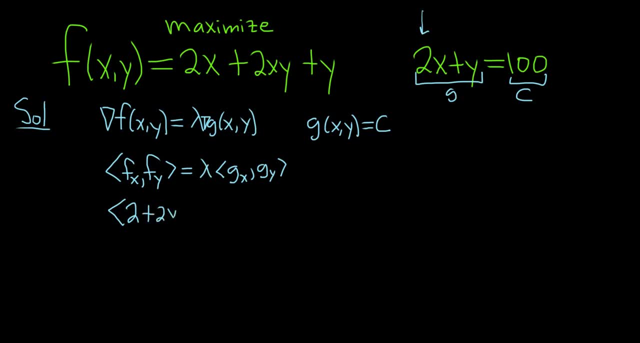 So we're just left with 2y, And the derivative of y is 0, so I won't bother to write it. So comma. Now we have to compute the partial derivative of f with respect to y. Well, the derivative of 2x is 0.. 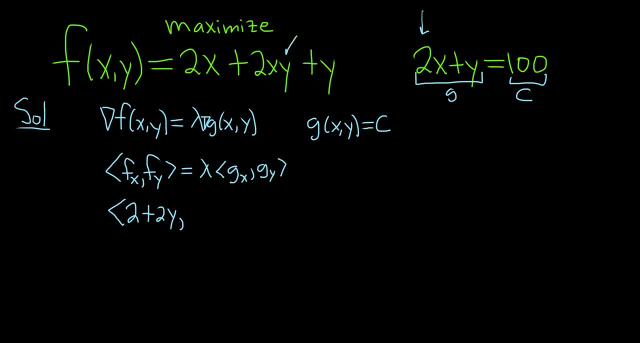 The derivative of 2xy. well, let's think about this: The derivative of y is 1, so we're just left with 2x, And the derivative of y is 1, so plus 1.. That's equal to lambda. 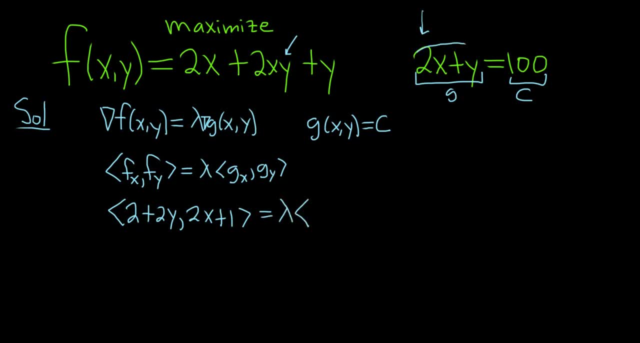 And then we have the partial derivative of g. This is always our g over here, so it's just going to be 2, right, Because the derivative of y is 0, and the derivative of 2x is 2.. And the partial derivative of g with respect to y is 1, right. 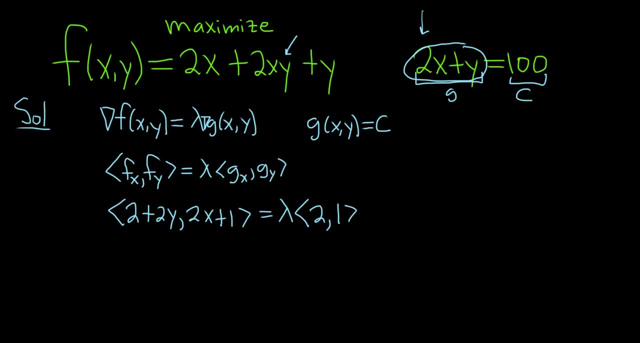 Because 2x that goes to 0.. Okay, so we did some math here. So we have 2 plus 2y comma, 2x plus 1. And then we have our angle bracket And that's equal to. 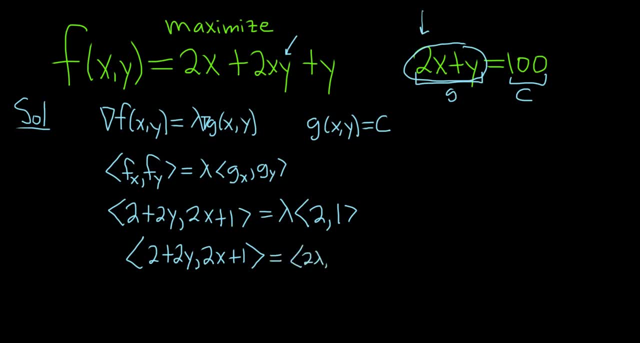 You can distribute the lambda. So this is 2 lambda. lambda, All right, good stuff. So these vectors are equal when their components are equal. So we'll take 2 plus 2y and set that equal to 2 lambda. 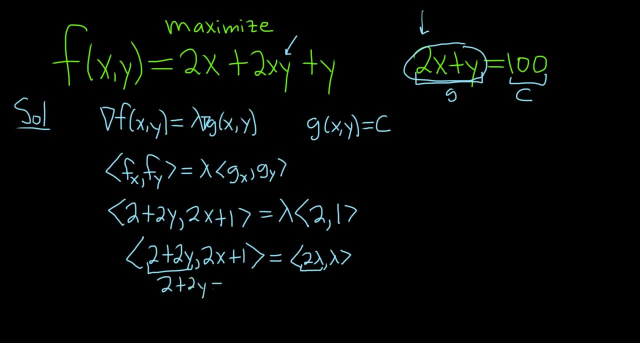 So 2 plus 2y is equal to 2 lambda. Okay, And then we'll take 2x plus 1 and set that equal to lambda. So 2x plus 1.. And that's equal to 2 lambda. 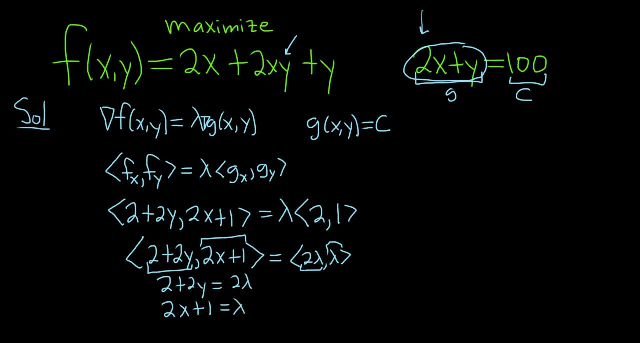 So how do you solve this? Well, it's up to you, but I'm a really big fan of matching, So we have like a 2 lambda here. It'd be really nice if this was also a 2 lambda. That way, we can set these equations equal. 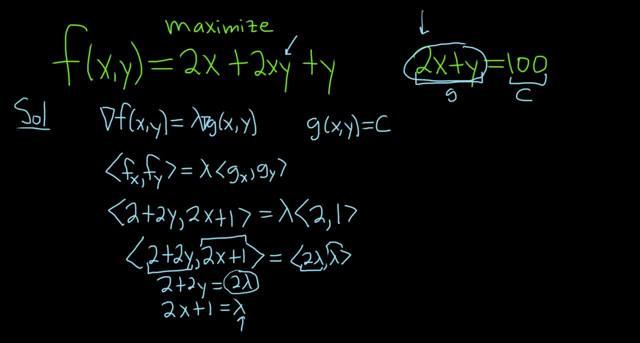 So what we can do is we can multiply the bottom equation by 2.. When we do that, we get 2 times 2x, so that's 4x, And then 2 times 1, which is 2.. And then we get it looks like 2 lambda right. 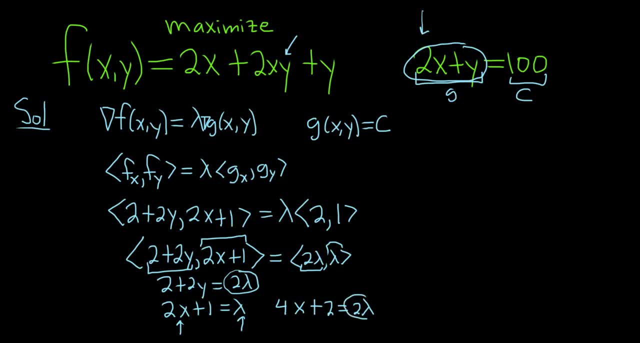 2 times lambda is 2 lambda. So this is also 2 lambda. So these are both 2 lambda. Therefore, 2 plus 2y must be equal to 4x plus 2.. So we can set these equal. 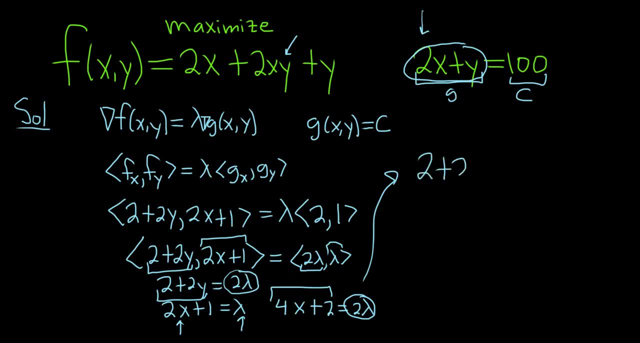 So we can set these equal. So we have 2 plus 2y equals 4x plus 2.. So again, it's a trick. So when you get here, you see the 2 lambda and you tell yourself: okay. 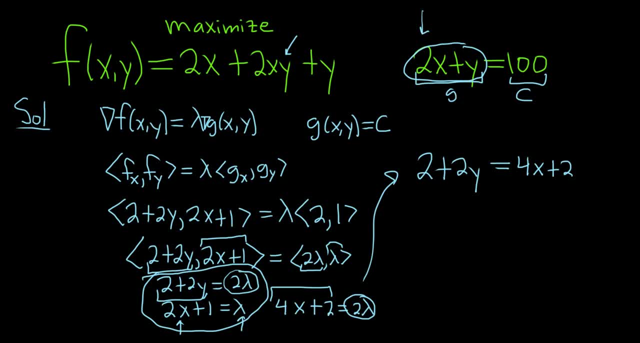 I want the lambda to be 2 lambda so I can set these equal. So you just multiply that second equation by 2.. It's super powerful And we did that, and then we can set them equal. Look, the 2s cancel. 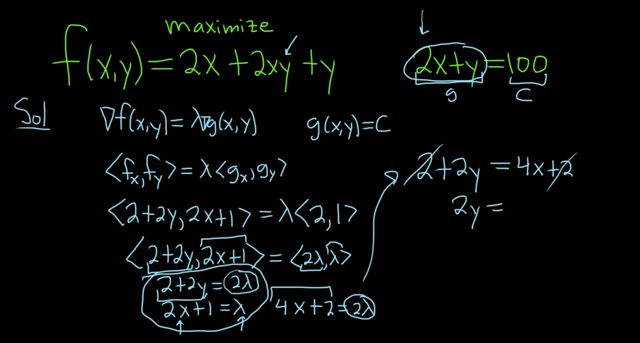 You can see, You can subtract them away. So we get 2y equals 4x. Dividing by 2 will give us y equals 2x, And we've reached a sticking point of sorts, right. So now we go back to our constraint. 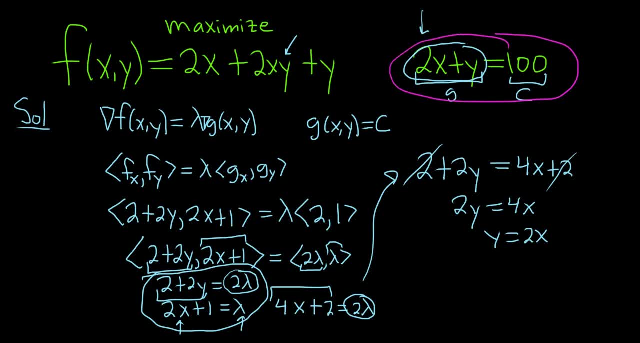 Our constraint is way up here. So 2x plus y is 100.. So we can replace the y with 2x, So this is 2x plus, and then y is 2x, so 2x And that's equal to 100. 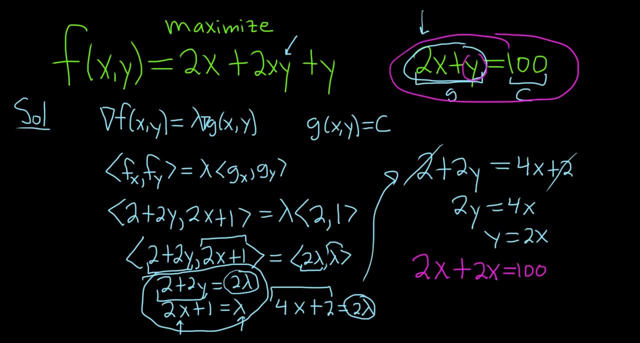 Yeah, I almost messed up there. It's really easy to mess up. So y is 2x, 2x plus 2x is 4x. Boom, That's equal to 100.. And then divide by 4.. 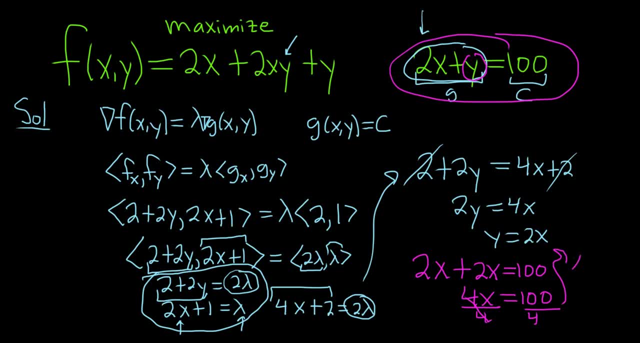 And hurrah. we have a value for x, which is really good. It means we're almost done, So x is 25.. Once we have x, we can plug it back in here, So we get y equals 2 times 25.. 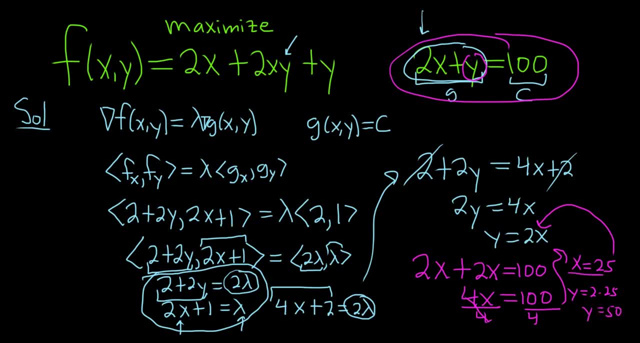 So y equals 50.. It's really good stuff. So we have x, We have y. Now all we have to do is plug it back into here And that will give us our maximum. So let's do it. So we have f of 25 comma 50.. 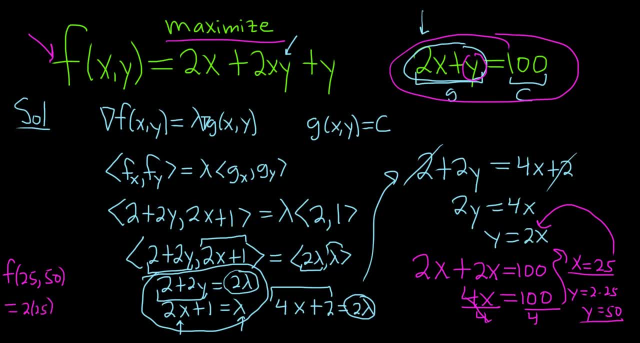 That's equal to 2 times 25 plus 2 times 25 times 50 plus 50.. And let me just double check this, Let me just see what it is. So it's 2 times 25 plus 2 times 25 times 50.. 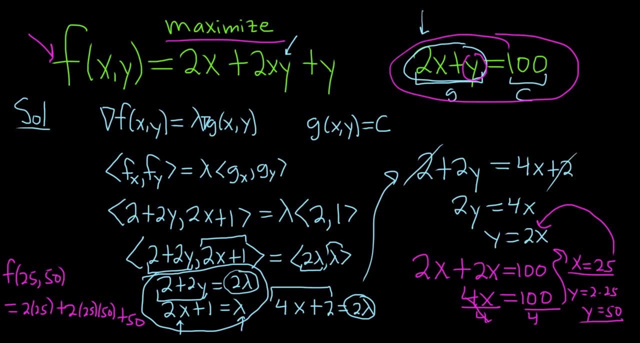 Tapping into my calculator, I got 2,600.. So 2,600 is the answer. So 2,600 is the maximum. So that's it. I hope this video has been helpful. 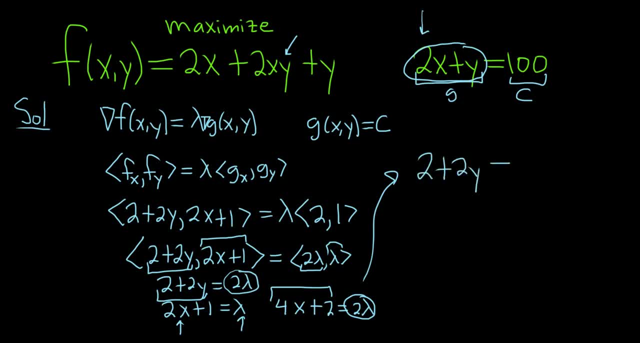 So we have 2 plus 2y equals 4x plus 2.. So again, it's a trick. So when you get here you see the 2 lambda and you tell yourself, okay, I want the lambda to be 2 lambda so I can set these equal. 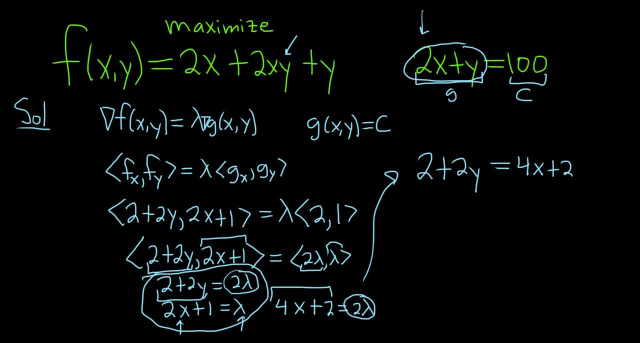 So you just multiply that second equation by 2. It's super powerful And we did that. and then we can set them equal. Look the 2s cancel, You can subtract them away. So we get 2y equals 4x. 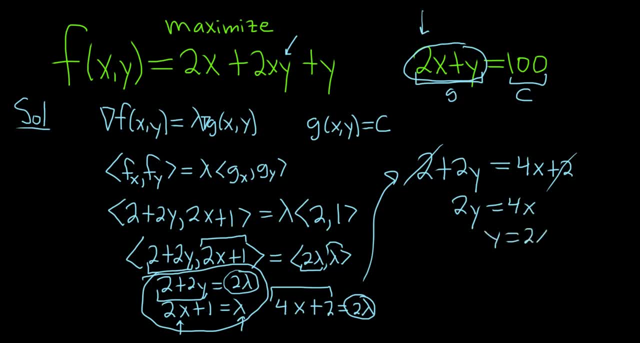 Dividing by 2 will give us y equals 2x, And we've reached a sticking point of sorts right. So now we go back to our constraint. Our constraint is way up here, So 2x plus y is 100. 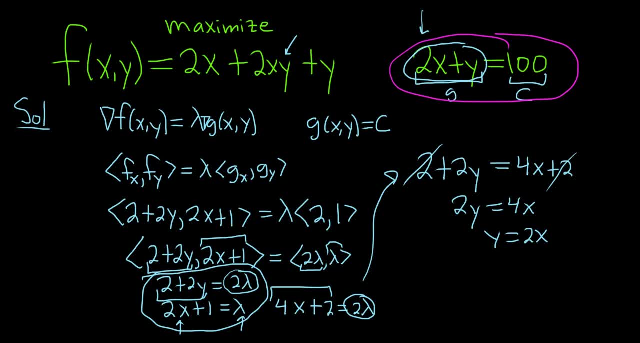 So we can replace the y with 2x, So this is 2x plus, and then y is 2x, So 2x, So 2x, And that's equal to 100.. Yeah, I almost messed up there. 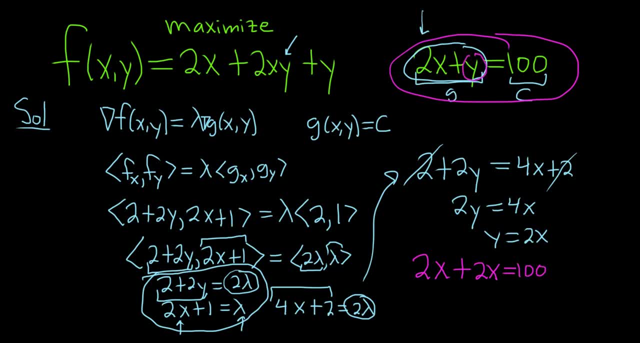 It's really easy to mess up. So y is 2x, 2x plus 2x is 4x. Boom, That's equal to 100.. And then divide by 4, and hurrah, We have a value for x, which is really good. 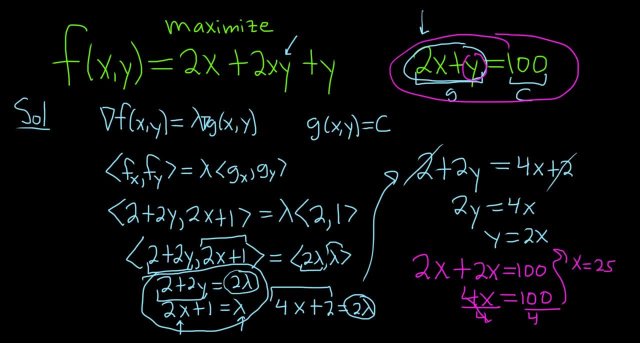 It means we're almost done. So x is 25.. Once we have x, we can plug it back in here. So we get y equals 2 times 25.. So y equals 50. It's really good stuff. So we have x. 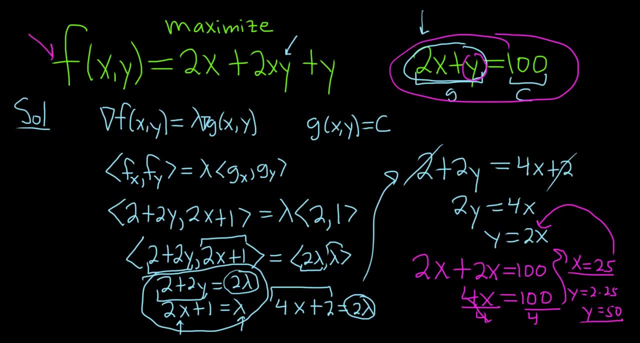 We have y Now. all we have to do is plug it back into here, and that will give us our maximum. So let's do it. So we have f of 25 comma 50. That's equal to 2 times 25 plus 2 times 25 times 50 plus 50.. 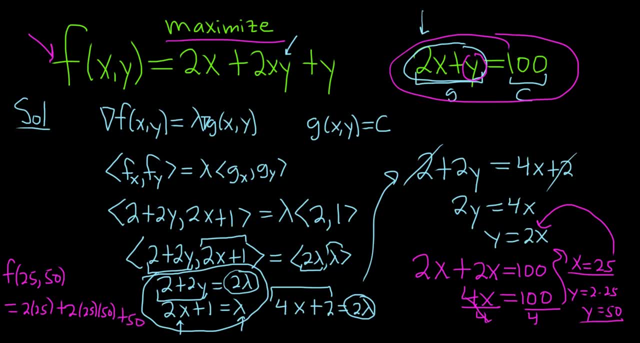 And let me just double check this. Let me just see what it is. So it's 2 times 25 plus 2 times 25 times 50. Tapping into my calculator, I got 2,600.. So 2,600 is the answer. 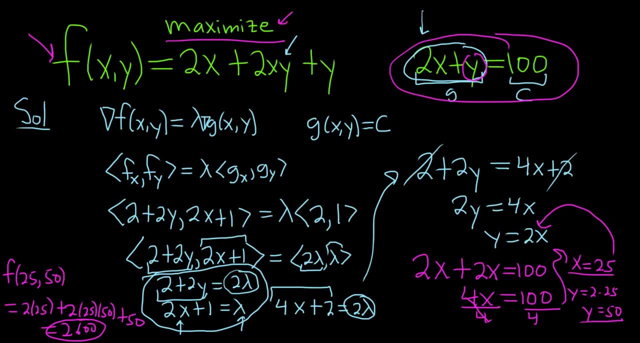 So 2,600 is the maximum. So that's it. I hope this video has been helpful.